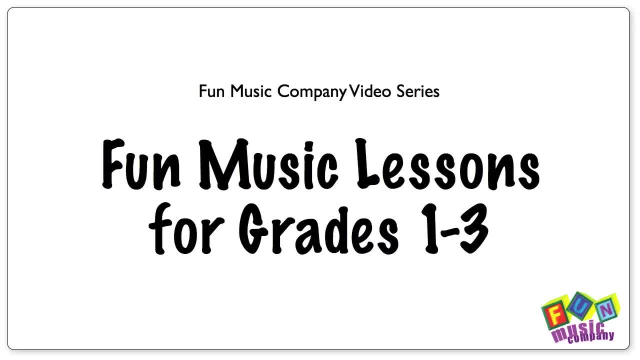 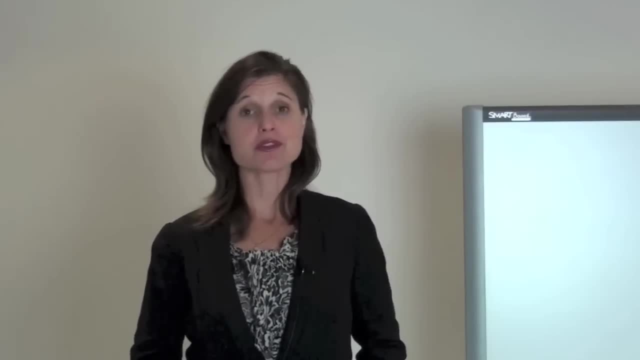 Hi, it's Janice Tark here from The Fun Music Company and today I've got an extra special activity to share with you from our whiteboard music lessons program for grades one to three, called Introduction to Music. Now you know I've had a great many discussions with teachers. 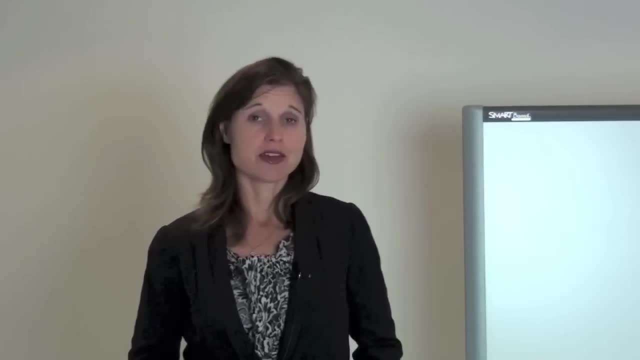 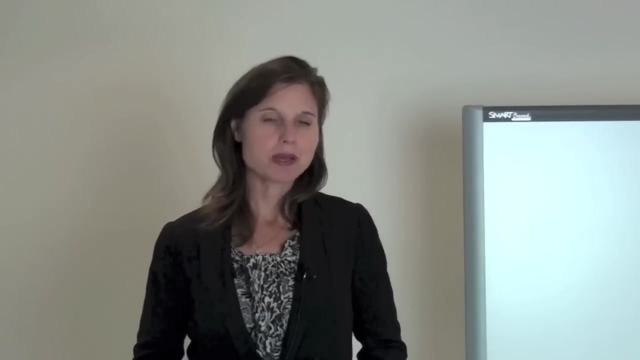 about what really makes something interactive, and do you know my answer? My answer is that an interactive activity is one where students do something rather than passively watch or listen. For this reason, a video played on an interactive whiteboard is not an interactive activity. 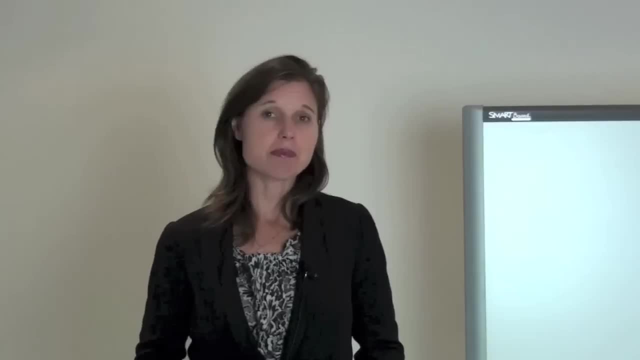 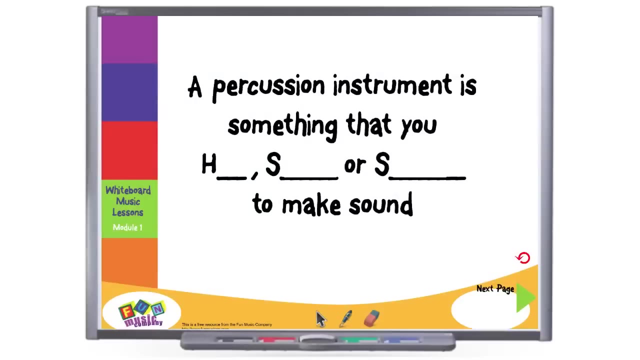 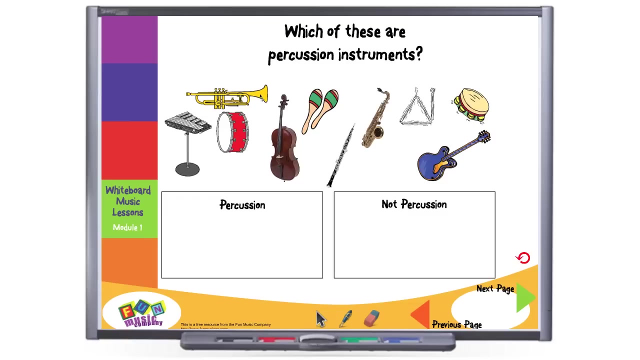 However, something where students are playing or singing is, For example, in today's sample resource, which comes from lesson four of Introduction to Music. the children will first define a percussion instrument as something that they can hit, scrape or shake to make the sound. Then, on this next slide, they can discuss various instruments and decide. 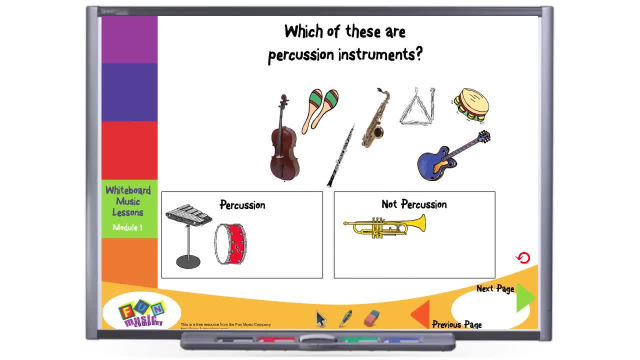 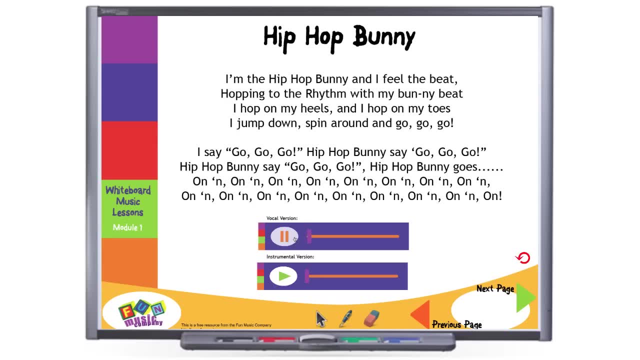 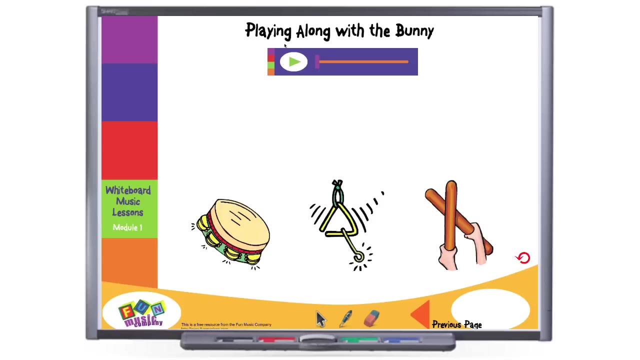 whether or not they fall into the category of percussion instruments. Then they can go ahead and get into some music, Now with our hip hop bunny song. this is a great little song and kids really do enjoy getting into it. On the next slide you can get out some instruments and you can play along Depending on their 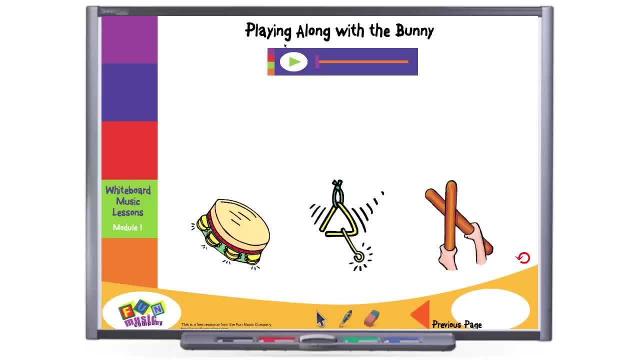 ability levels. there are a lot of choices of what rhythm to play, and as there is nothing on the actual slide except for the music, then as a teacher you can go ahead and make those choices. Here are a few ideas. Here are a few ideas.